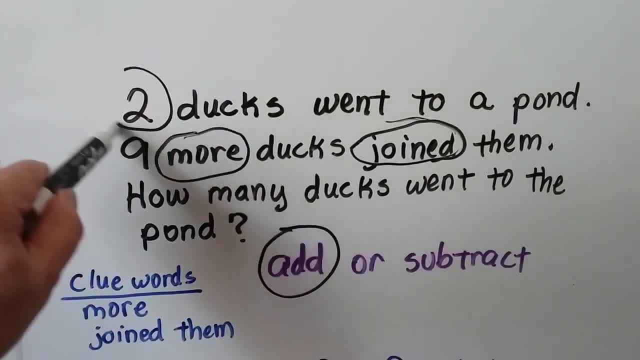 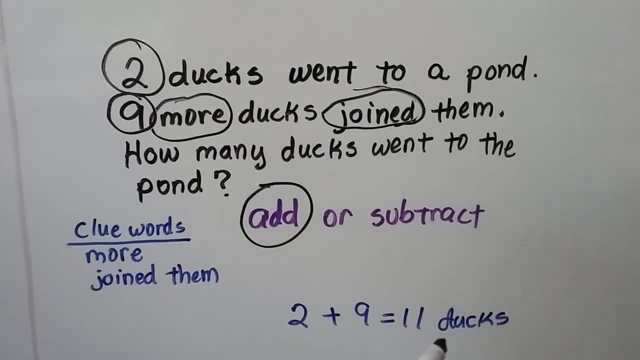 do. addition, We're going to circle our important numbers. Nine more ducks joined them, So we're going 2 and 9.. We're going to add them. 2 plus 9 is 11 and we label it as ducks. It's 11. 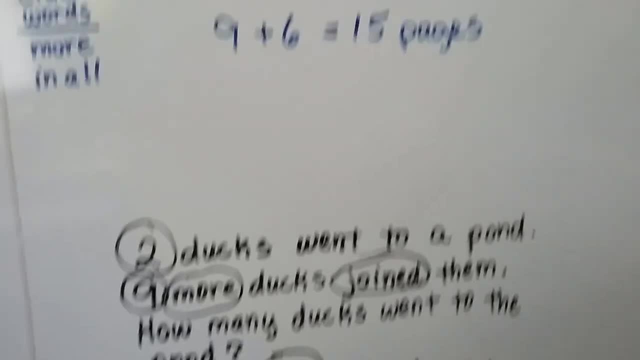 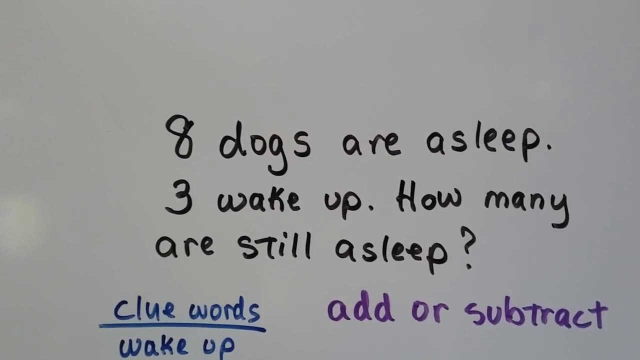 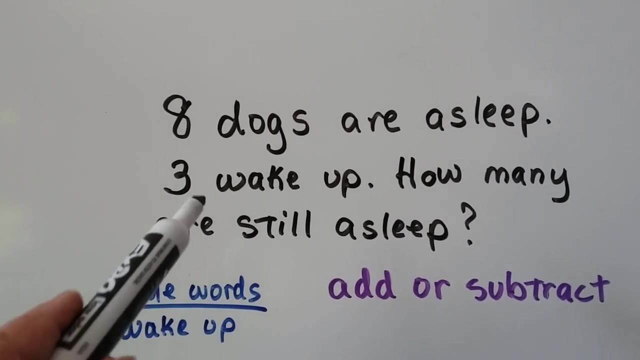 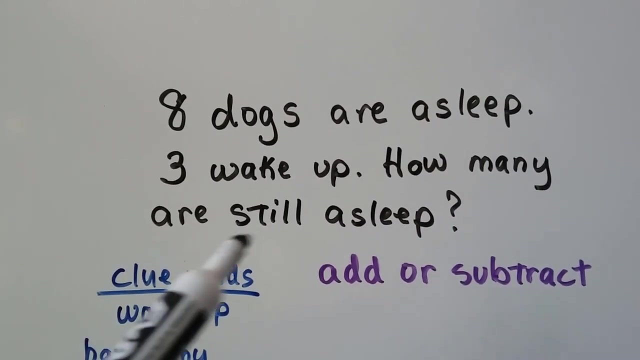 ducks. Let's try another one. We have eight dogs are asleep, Three wake up. How many are still asleep? Our clue words are: wake up and how many are still So it says that eight were asleep, but three wake up. This is a subtraction sentence. 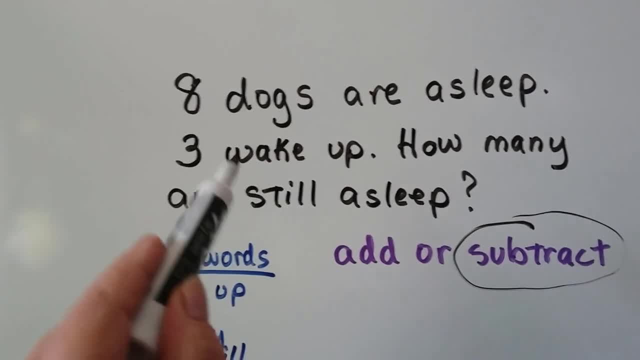 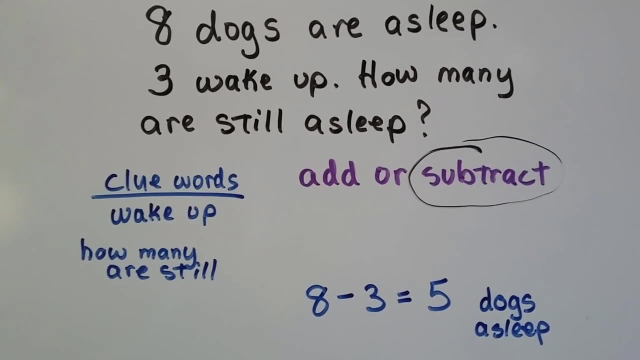 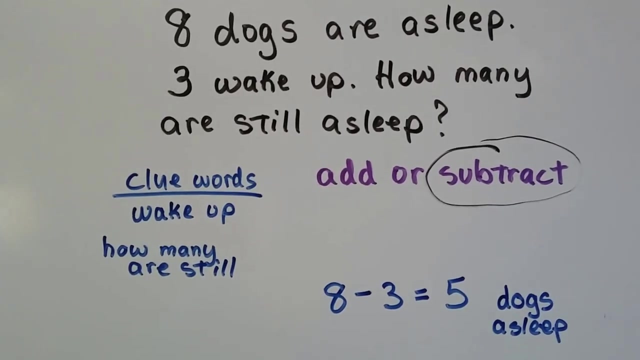 We need to subtract the three that woke up from the eight, So we do 8 minus 3 equals 5 dogs asleep. See, it told us we needed to find the ones that were still asleep. Let's try this one: Four monkeys eat. 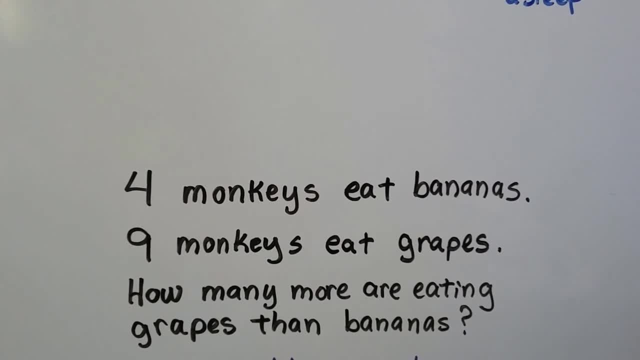 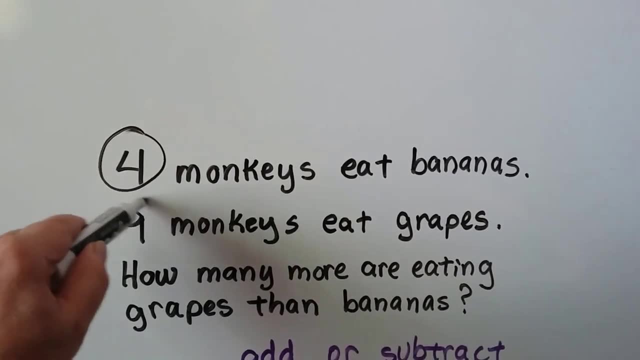 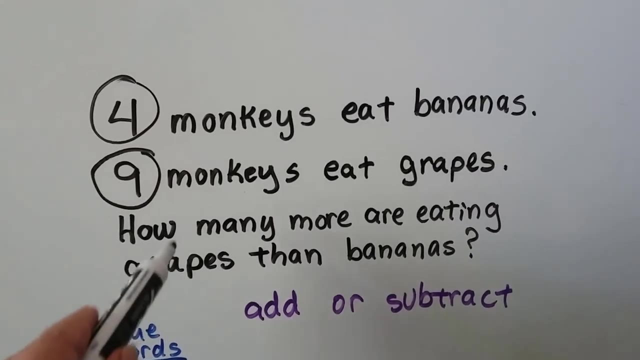 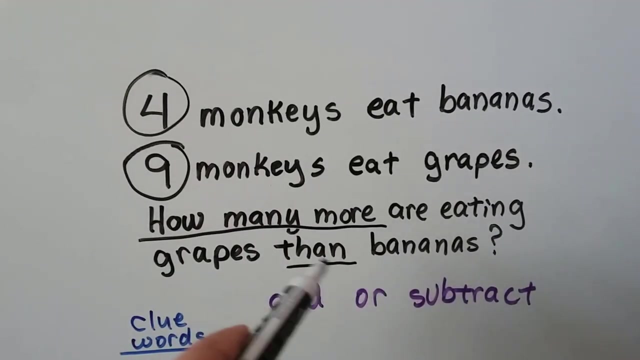 bananas. Nine monkeys eat grapes. How many more are eating grapes than bananas? Well, we circle important numbers. Look for our clue words. Our clue words are: how many more and than It says? how many more are eating grapes than bananas? So we need to. 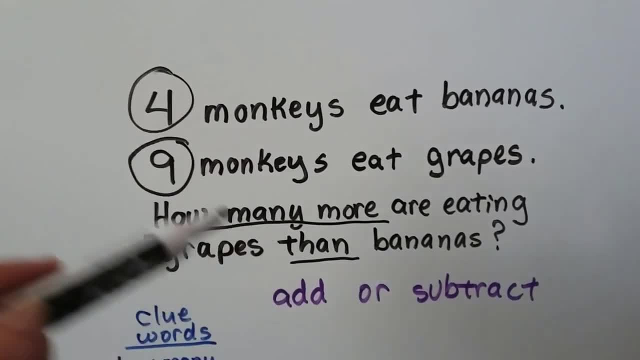 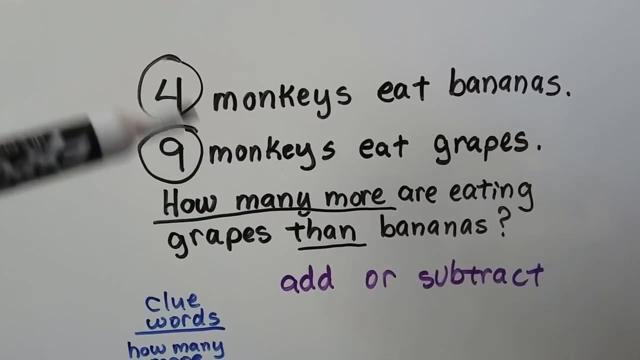 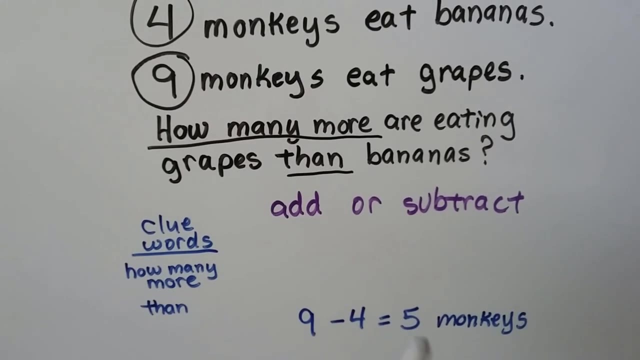 find the difference between grapes and bananas. Well, four were bananas and nine were grapes. We need to find the difference between these two numbers, And the bigger number is the minuend. That's gonna go first. 9 minus 4 equals 5.. And 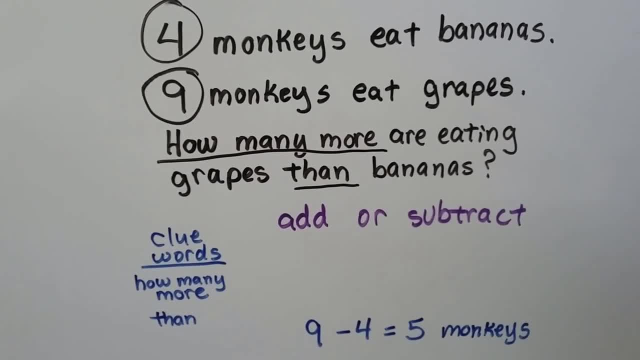 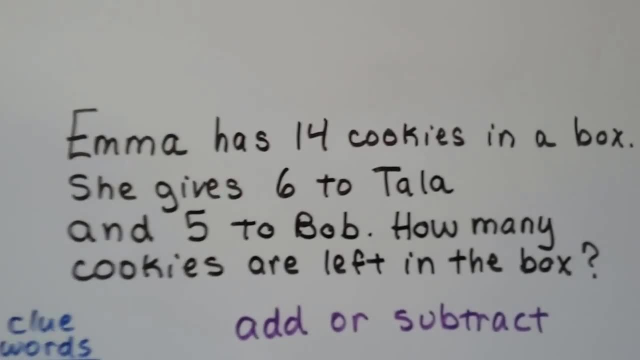 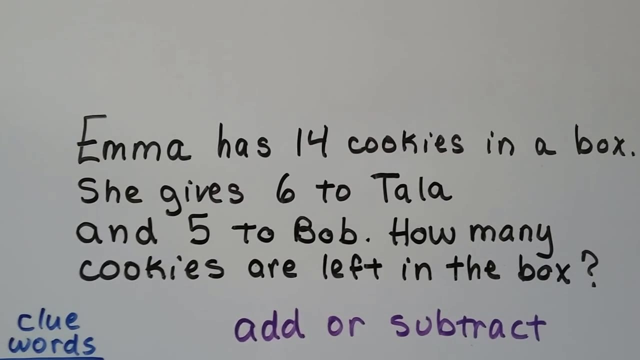 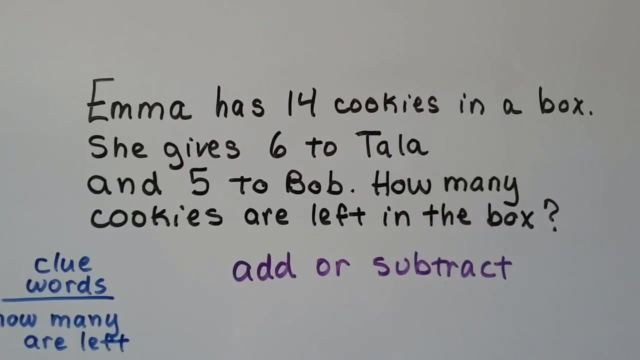 five more monkeys are eating grapes than bananas. Let's try this one. Emma has 14 cookies in a box. She gives six to Tala and five to Bob. How many cookies are left in the box now? there's a couple ways we can solve this. we